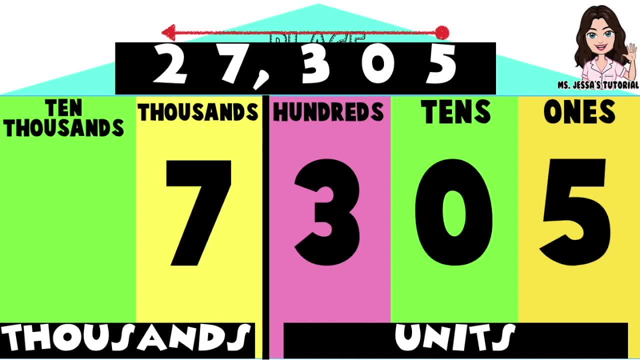 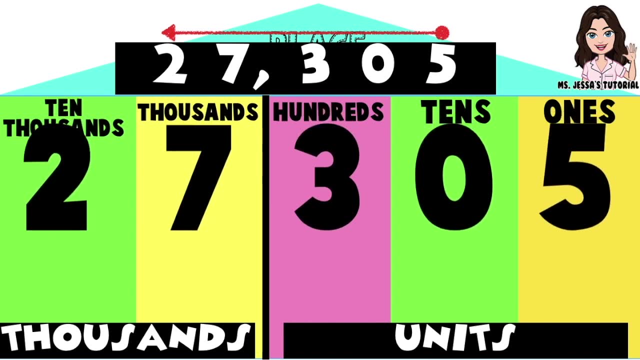 So digit seven will be in the thousand's place. And lastly, the fifth digit from the right is digit two. Digit two is in the ten thousand's place. So these are the place value of the digits in twenty-seven thousand three hundred five. 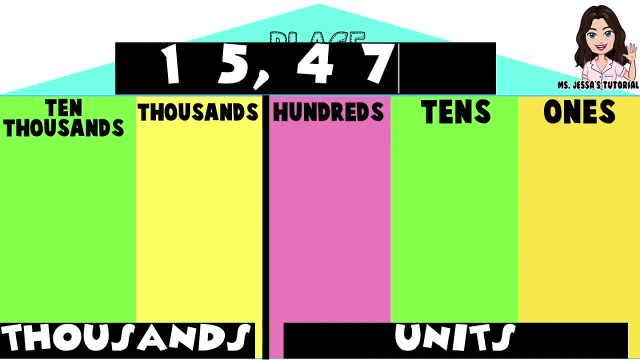 Let's have another example. Fifteen thousand four hundred seventy-four Again, children. in identifying the place value, you are going to start from the rightmost digit, going to the leftmost digit. Digit four is the first digit from the right. 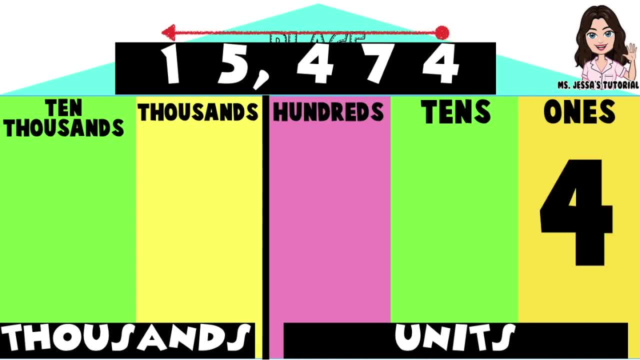 So digit four is in the one's place. Next is digit seven, Since digit seven is the second digit from the right. So digit seven is in the tenth's place. Next is digit four. Digit four is the third digit from the right. 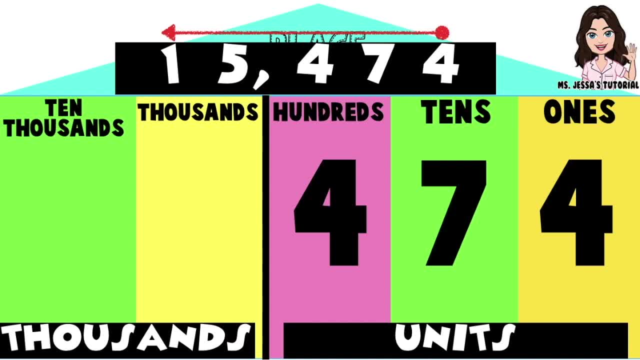 So digit four is in the hundred's place, Then next is digit five, Digit five is in the thousand's place And lastly, digit one is in the ten thousand's place place. so these are the place value of the digits in 15474. how about if we? 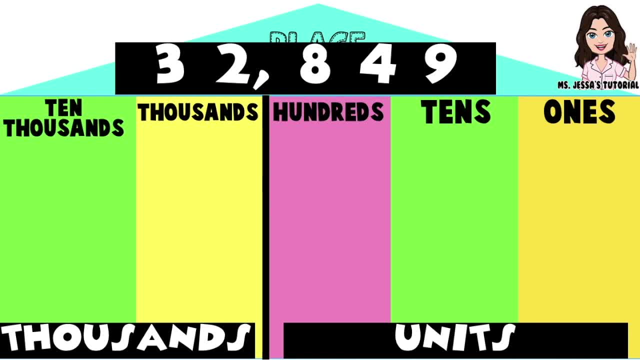 have 32,849 again. children, in identifying the place value, you are going to start from the rightmost digit, going to the leftmost digit. let's start at digit 9. digit 9 is the first digit from the right, so the place value of digit 9 is once. digit 4 is the second digit from the right and its place value. 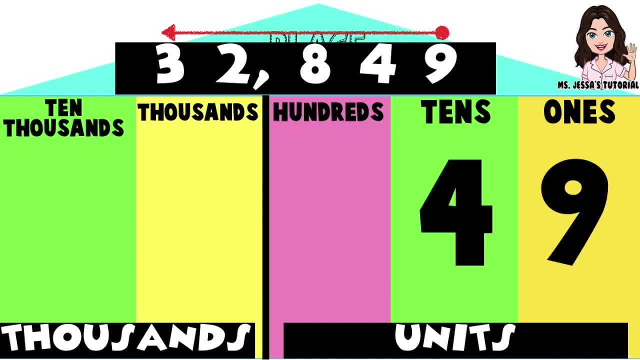 is tense. digit 8 is the third digit from the right and its place value is hundreds. digit 2 is the fourth digit from the right, is yeah digit from the right and its place value is thousands. And digit 3 is the 5th digit from. 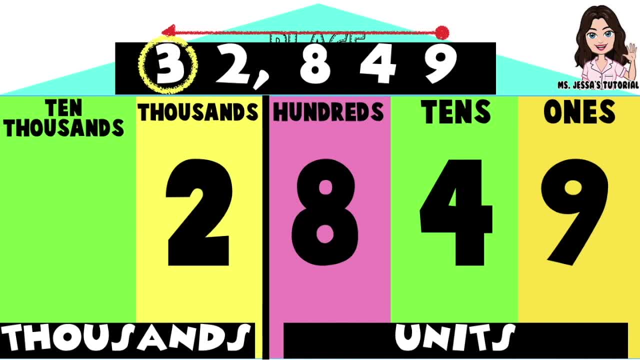 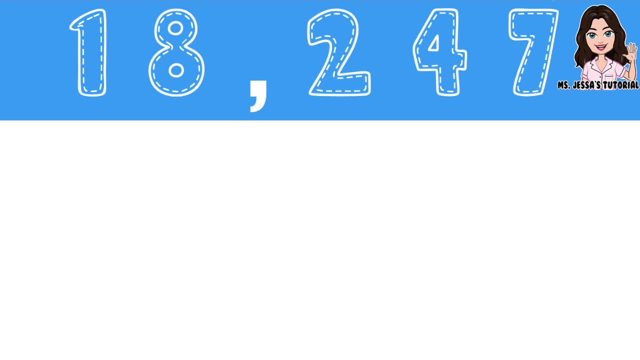 the right and its place value is ten thousands. So these are the place value of digits in 32,849.. What if we have 18,247?? Again, children, in identifying the place value you are going to start from the rightmost digit going to the leftmost digit. Digit 7 is one's place. 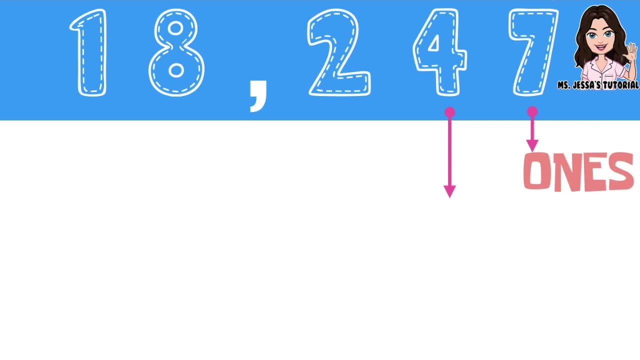 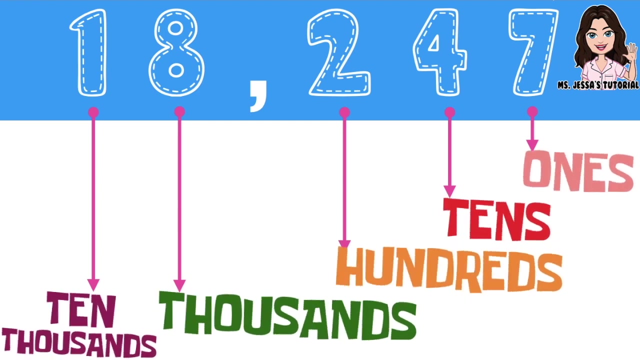 Digit 4 is 3rd 10's place, Digit 3 is 100's place, Digit 8 is 1000's place, While digit 1 is 10,000's place. So these are the place value of 18,247.. 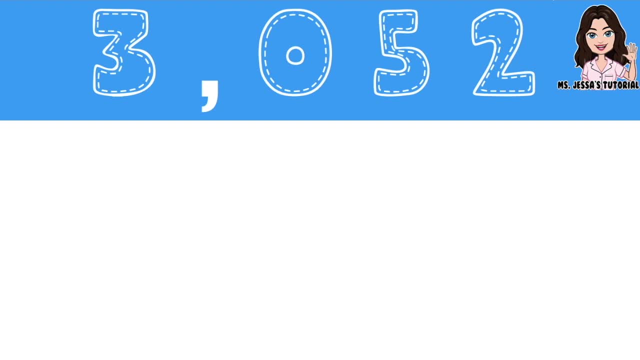 How about if we have 3,052?? Again, children, in identifying the place value, you are going to start from the rightmost digit, going to the leftmost digit. Digit 2 is 1's place. Digit 5 is 10's place. 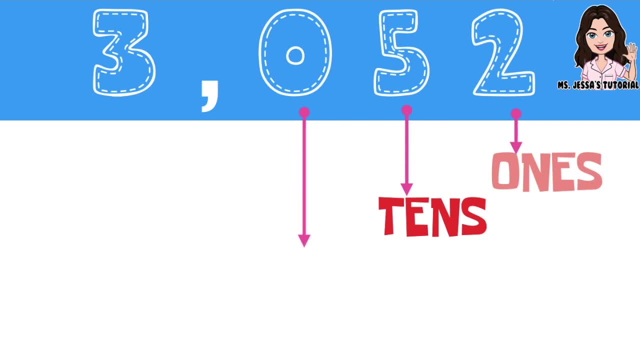 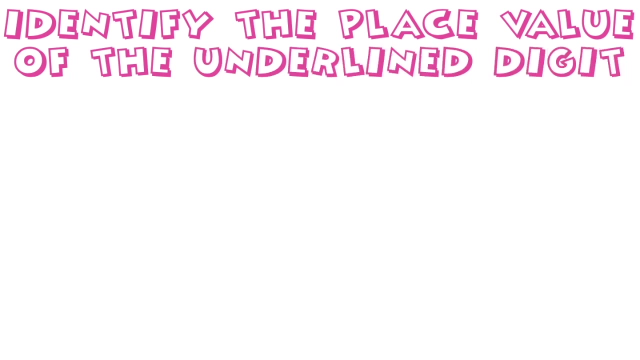 Digit 0 is 100's place, While digit 3 is 10,000's place. These are the place value of digits in 3,052.. So now you are ready to identify the place value of the underlined digit. 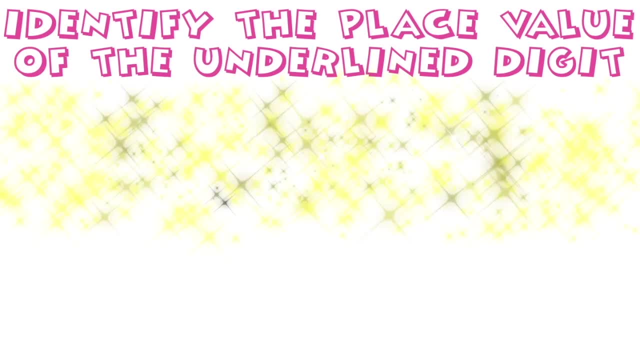 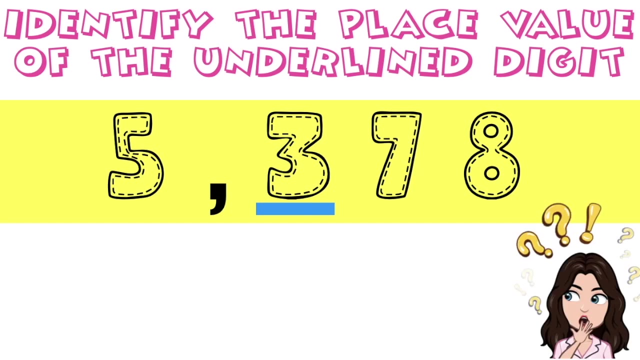 Let's have the first example, 5,378.. What is the place value of digit 3?? Again, children, in identifying the place value, you are going to start from the rightmost digit, going to the leftmost digit. Digit 8 is ones. 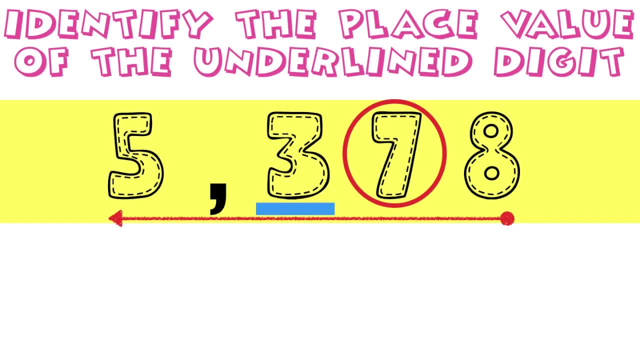 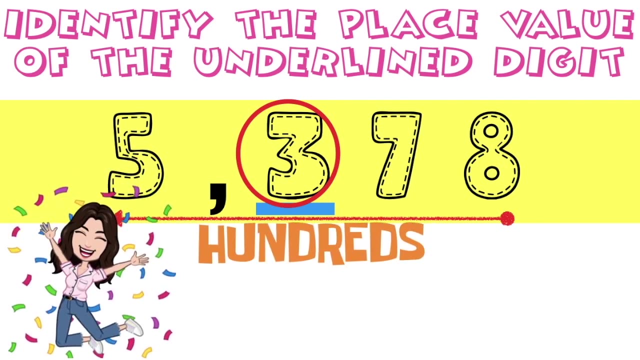 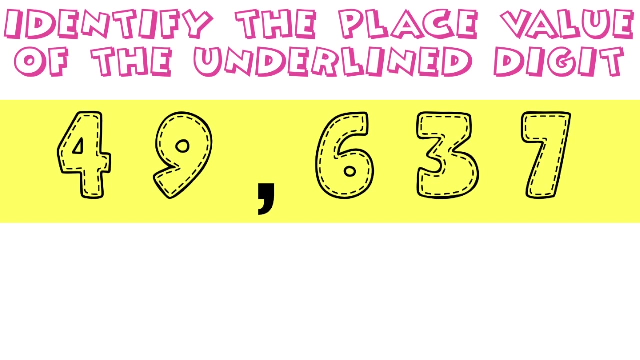 Digit 7 is tens, So therefore digit 3 is hundreds. Very good, How about if we have 49,637? Let's identify the place value of digit 4. Again, children, in identifying the place value, you are going to start from the rightmost digit, going to the leftmost digit. 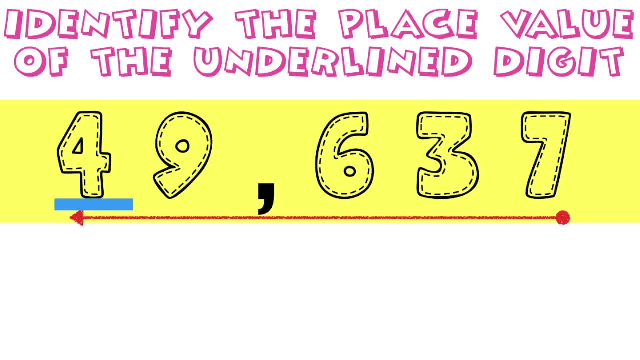 Let's start. Digit 7 is ones, Digit 3 is tens, Digit 6 is hundreds. Digit 9 is thousands And finally, digit 4 is- I can't hear you what is it? Digit 4 is ten thousands. Good job. How about if we have this one? 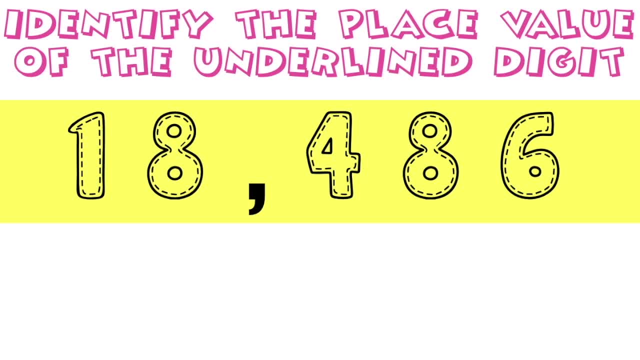 18,486. What is the place value of digit 8?? Again, children, in identifying the place value, you are going to start from the rightmost digit, going to the leftmost digit. Digit 6 is hundreds. Digit 7 is hundreds. Digit 6 is. 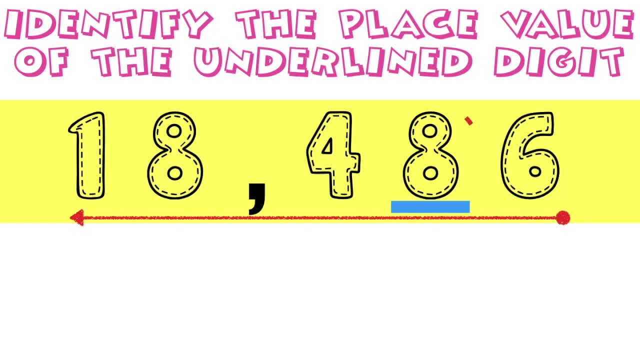 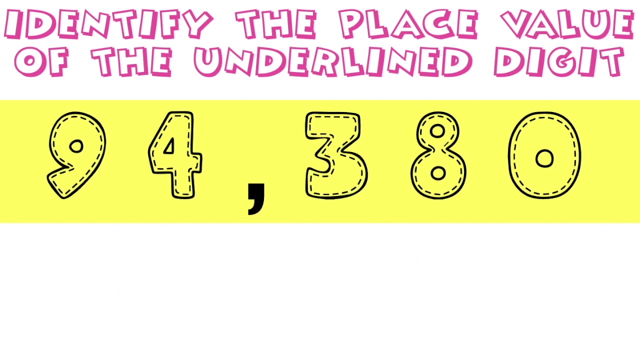 D distracted One As it was before that it was divided into one and two. What is digit 8?? Digit 2 is hundreds. So what is digit 8?? 14,316 очка. When it is a Wants, What is the place value of digit 8?? 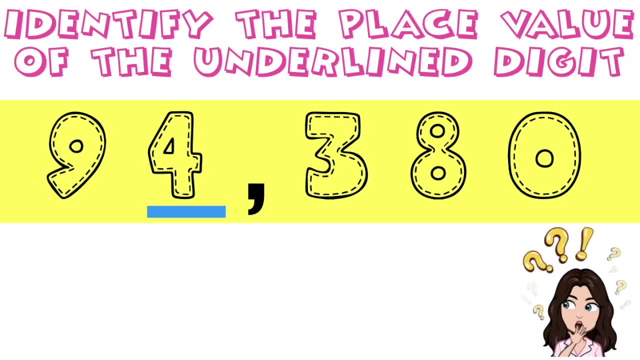 Thanks for watching value of digit 4.. Always remember, in identifying the place value, you're going to start from the rightmost digit, going to the leftmost digit. So let's start. Digit 0 is ones, Digit 8 is tens, Digit 3 is hundreds. So how about digit 4, children? Can I hear your voice Louder? 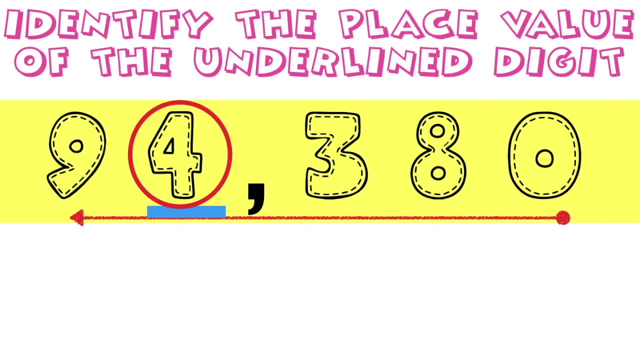 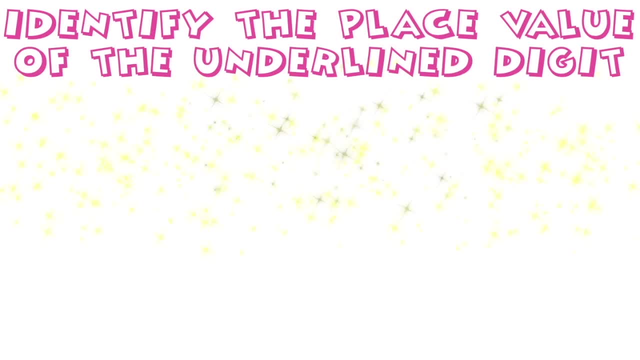 I can't hear you. Digit 4 is thousands. Very good, How about if we have this one, 709.. What is the place value of digit 9?? So always remember, in identifying the place value, you're going to start from the rightmost digit going to the leftmost digit. So since digit 9 is the 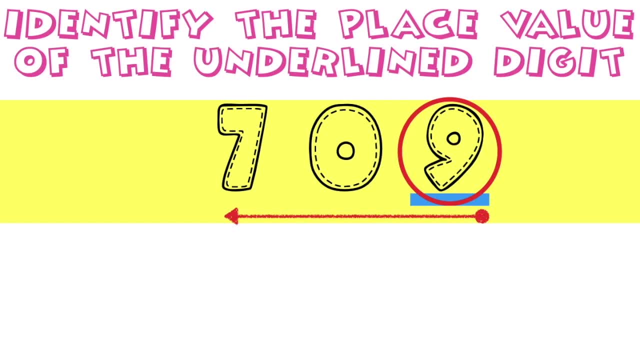 first digit from the right. so what is the place value? I can't hear you. What is the place value of digit 9?? What is the place value of digit 9?? True, Precisely, Digit 9 is in the ones place. 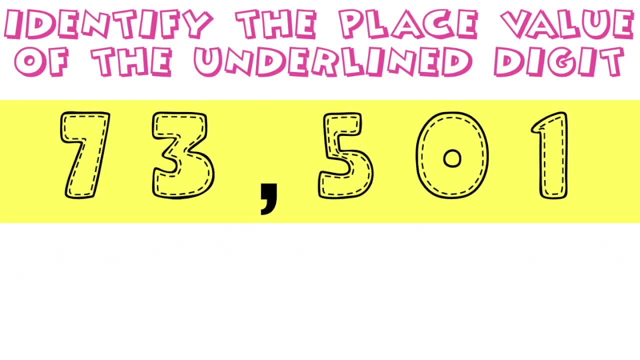 Let's have our last example. Seventy three thousand five hundred one, What is the place value of digit 7?? Again, children, In identifying the place value, you're going to start from the rightmost digit, going to the leftmost digit. So, since both places belong to the when, so whatever the value is, you're going to start from the rightmost digit, going to the leftmost digit. Yeah, Let's try the fields. One place value is the seventh, which is what It's aancing plus seven. إ pris 1958: शупि�� ऑ किति भी discord, 197. 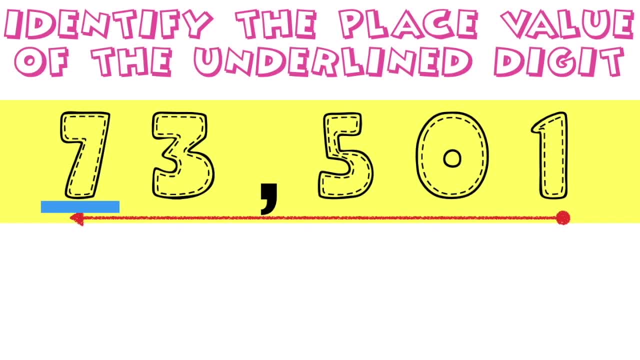 You'll be left-side digit 8 healthy n것도. okay. now the person who's right side digit 8 will start from the leftmost digit. going to the leftmost digit HTML. today You can see that people start NASA. yet let's start. digit 1 is ones. digit 0 is tens. digit 5 is hundreds. digit 3 is: 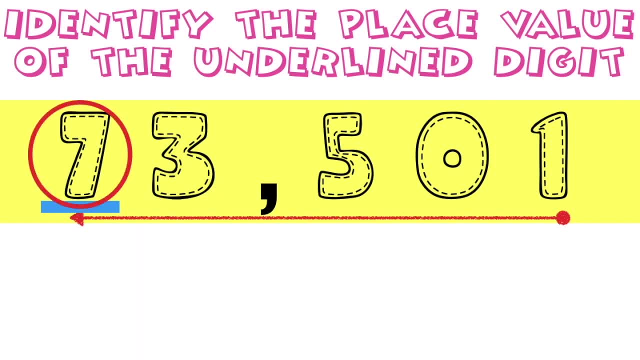 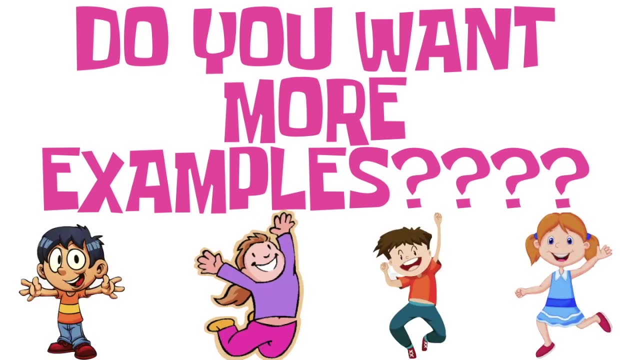 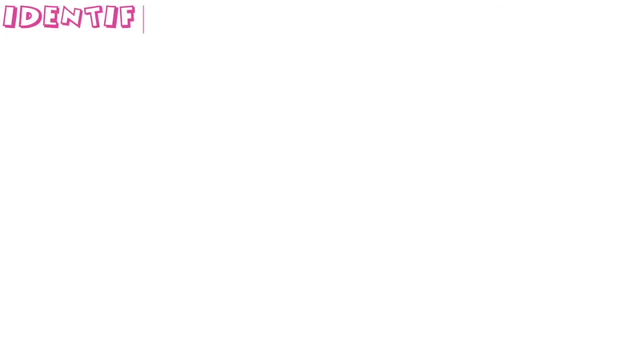 thousands and digit 7 is ten thousands. very good, do you want more examples? okay, your wish is my command. let's have more examples here. let's identify the digit in the number that has the given place value: 23 sixths thousand nine twenty three thousand six hundred ninety four. what is the digit? 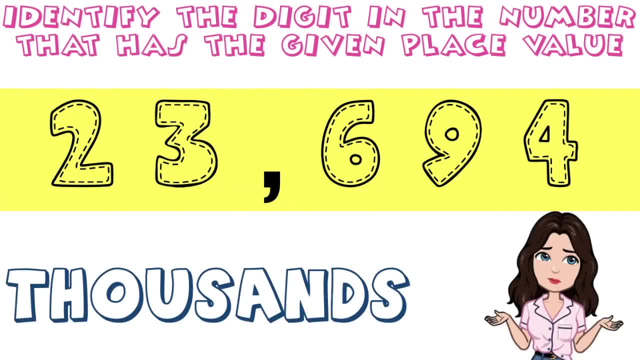 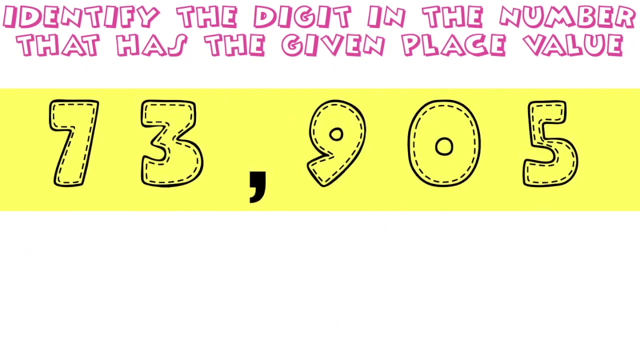 in the thousands, please let's start ones. tens, hundreds thousands. so digit three is in the thousands. let's check then. how many people are there five, six? How about if we have 73,905?? What is the digit in the ten-thousandths place? 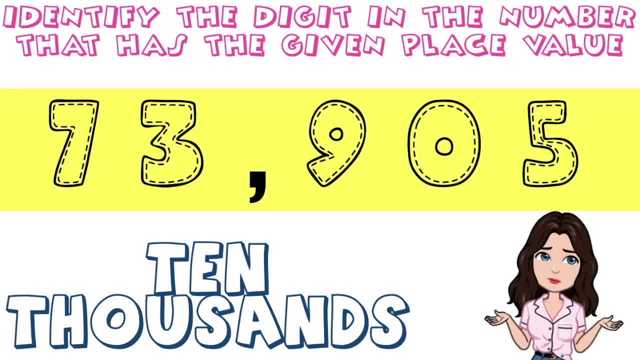 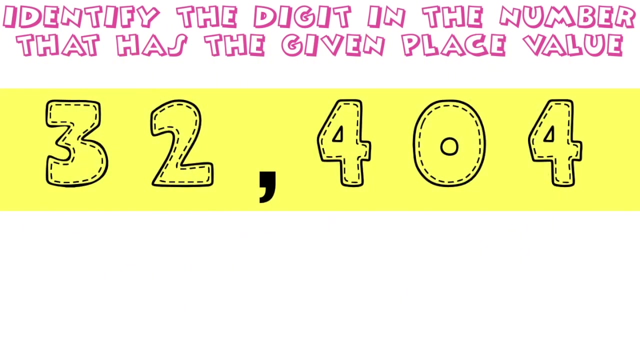 Let's do it together. Speak louder. Let's start. Ones, tens hundreds thousands, ten-thousands. So digit seven is in the ten-thousandths place. How about if we have 32,404?? What is the digit in the ten-thousandths place? 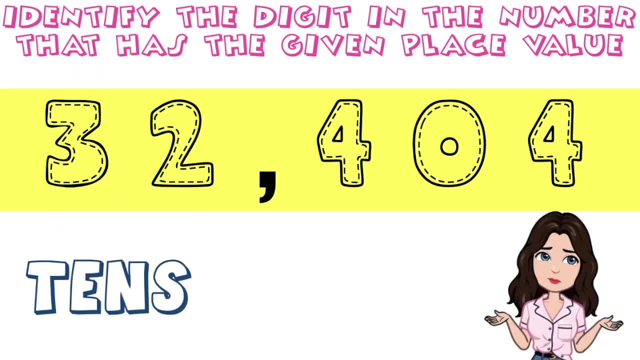 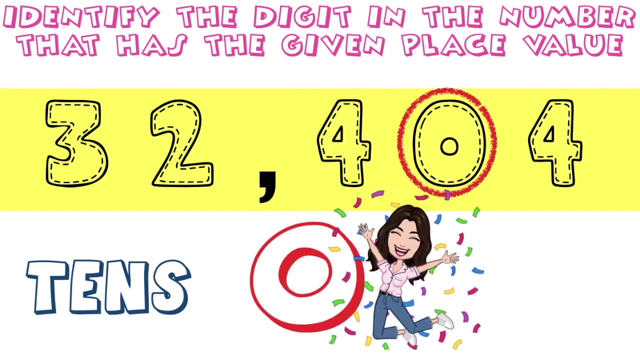 What is the digit in the ten-thousandths place? Let's do it together. children Speak louder. Let's start Ones, tens. So digit zero is in the ten-thousandths place. How about if we have this one? 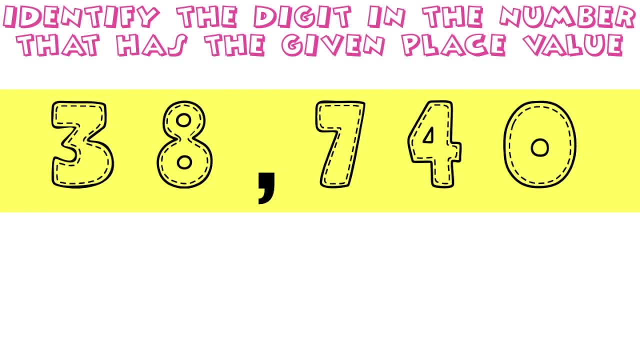 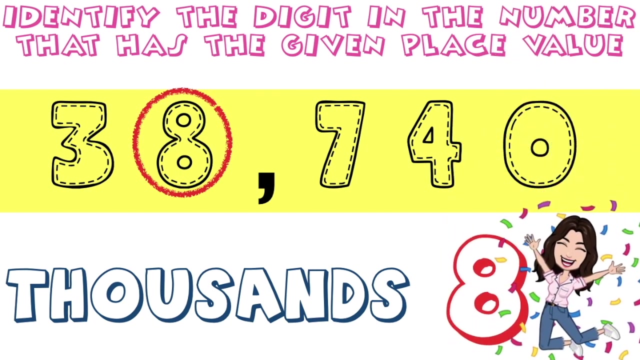 38,740.. What is the digit in the ten-thousandths place? Let's do it together: Ones tens hundreds thousands. So digit eight is in the ten-thousandths place. Let's have our last example. 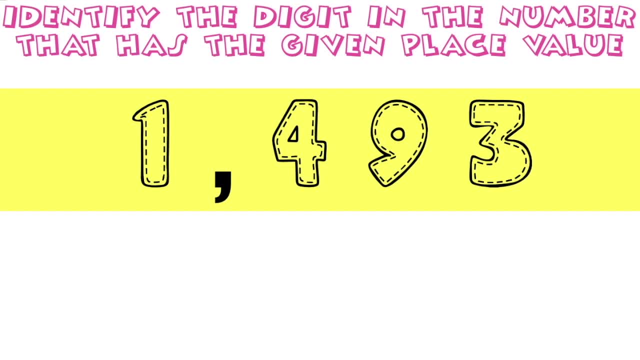 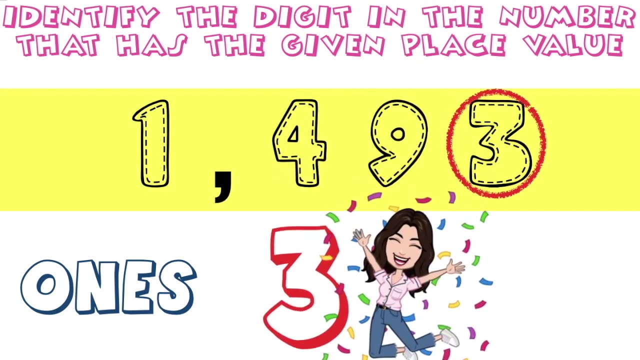 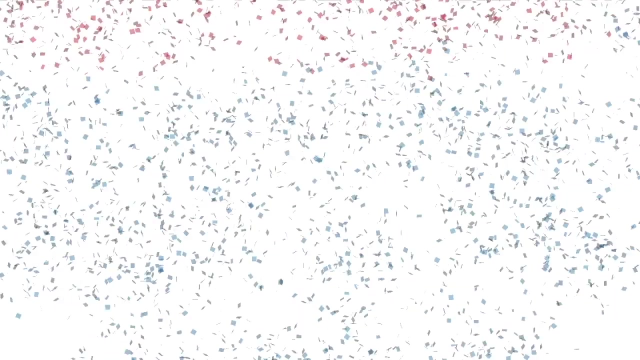 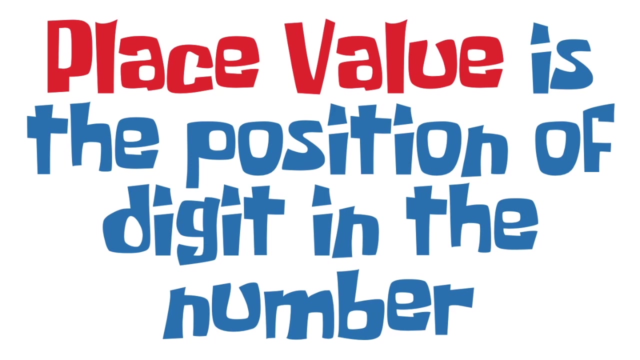 One-thousand four-hundred-ninety-three. What is the digit in the ones place place? That's so easy. Once So, digit 3 is in the once place. What have you learned? Place value is the position of digit in the number. In a 5 digit number, the first digit,